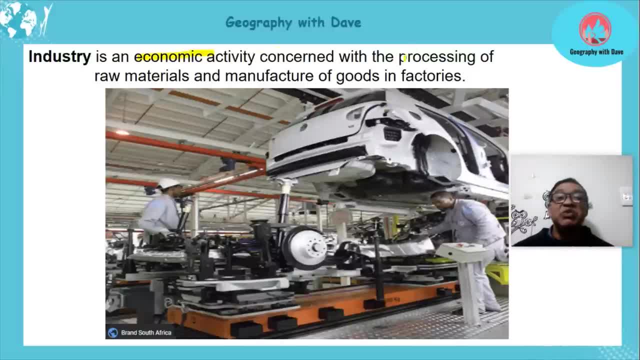 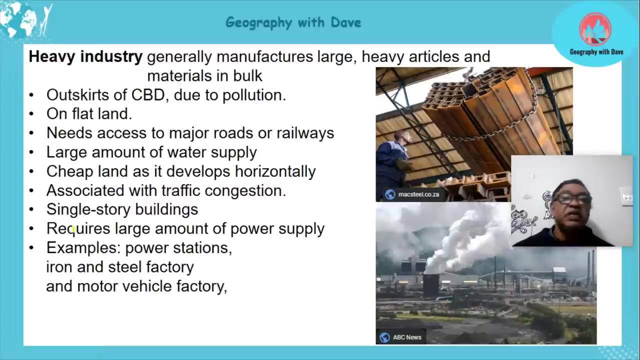 So it's an economic activity concerned with processing of raw materials and manufactured goods in places like factories, and not just factories, bakeries and whatever. Okay, So that is an industry. Okay, We start off. I know you have done these sort of things in your 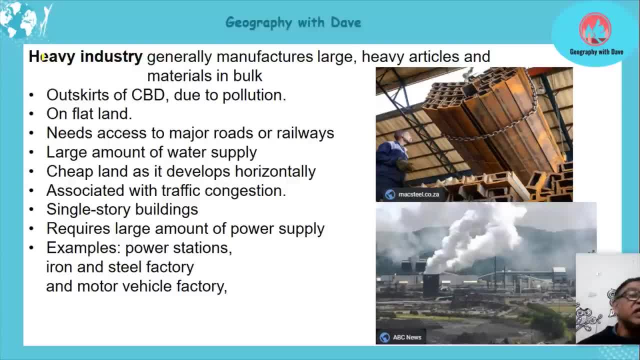 previous grades. but let's look at a heavy industry. All right, Now what is very known about it? It manufactures large heavy articles and materials in bulk. That's what it generally manufactures. Okay, You can see here the iron and steel. All right, You can see the horizontal space. 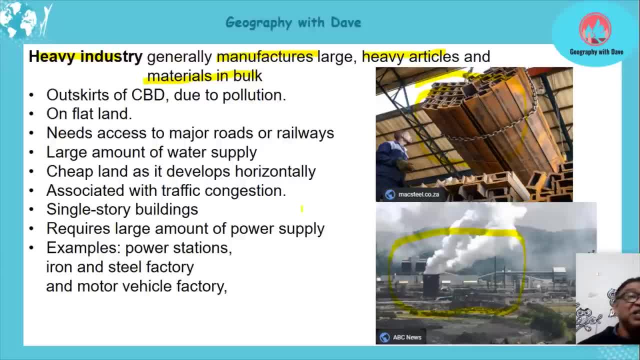 it occupies. It pollutes a lot also. So let's look at some of the characteristics of this heavy industry. It's on the outskirts of the CBD, due to the pollution. Imagine having this in the CBD, All right, Right in there. It's going to pollute the area. It's going to create too much of that sort of problem. 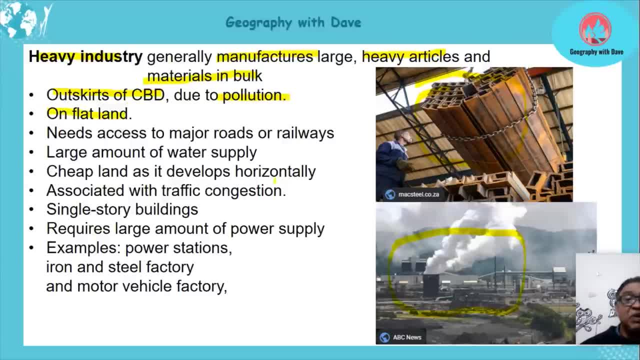 Okay, On flat land, because it develops horizontally. All right, Yeah, I guess I'll see that we'll talk about single-storey buildings later. All right, Because it's horizontal, it needs flatland and it deals with park goods etc. Okay, So you can't have it. 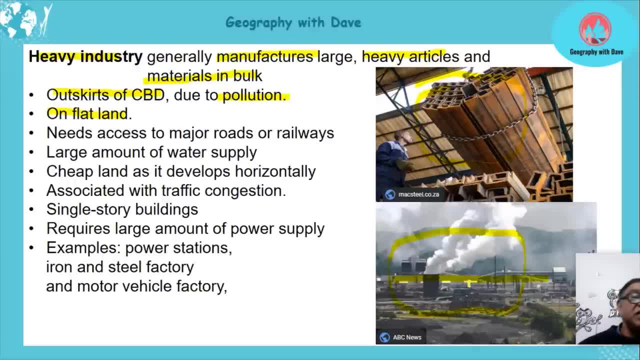 in an area which is very hilly Doesn't make sense. Needs access to major roads and railways. The bulk raw materials are coming in Right And the products which are bulky are going out, So you need these major roads to transport it. We are in a time when the power is running out. Railways. 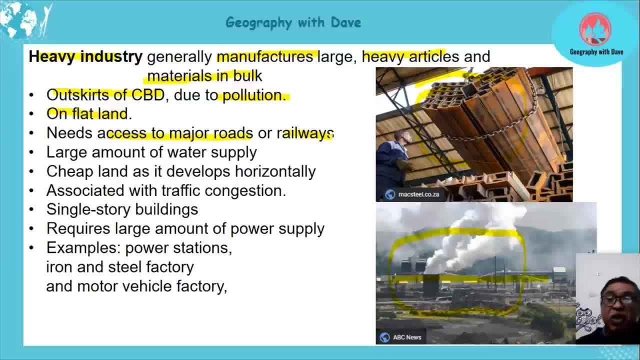 a cheaper form of transport. you need it around there, okay, in order to transport in and out of those industries. of course, it will use a larger amount of water supply, cooling systems, furnaces or washing of stuff. whatever massive right, it requires cheap land as it develops horizontally. 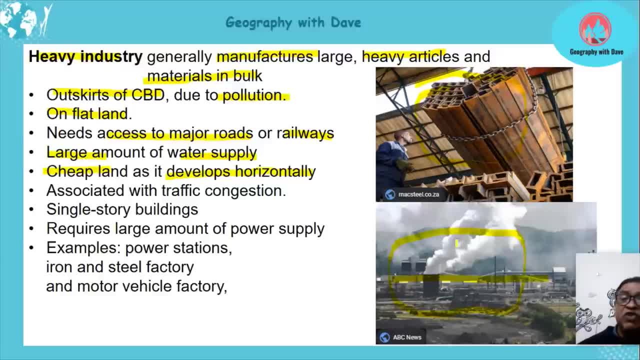 you can't have multi-story buildings here. so if you can occupy a large horizontal space and the land is very expensive, it'll create many challenges cost-wise for your industry. so cheaper land. that is why it's more towards the outskirts of the cbd etc. okay, it is associated. 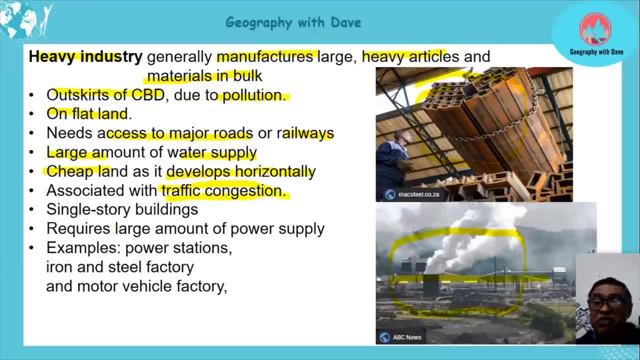 with traffic congestion, all right. don't say traffic traffic congestion, because there's a lot of trucks and materials coming in, etc. which is creating a lot of congestion. and, as i mentioned, single-story buildings and if you look at this, they are single story here- all right. you can't have multi-story. you can't carry bulk iron and steel up into multi-story. 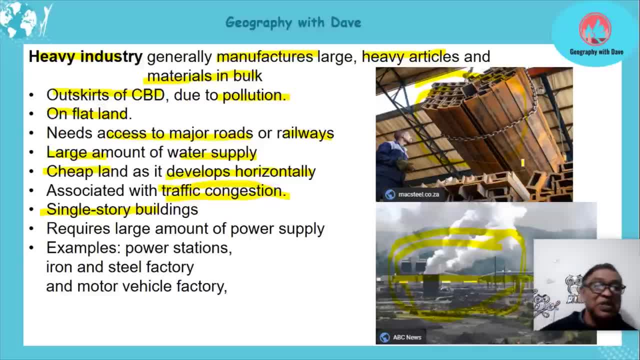 buildings doesn't make sense, all right. so the single story building it requires a large amount of power supply. if you look at this, iron and steel, it must be smelted or melted, whatever you understand, at high temperatures. the power, that gen that's used up in all this to manufacture cars, to do this, all right, it's huge. okay, one of the examples: 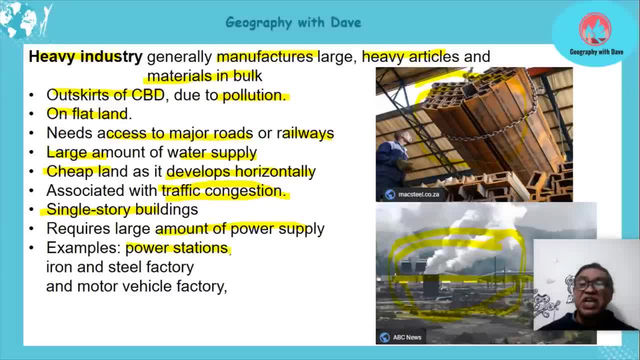 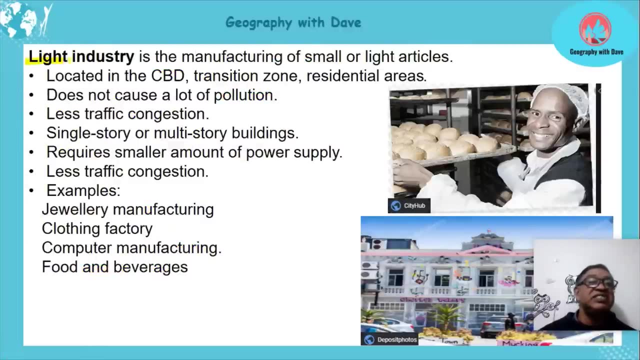 power stations, who sort of create electricity, iron and steel factories, motor vehicle factories- these are heavy industries that you would get. all right, let's go on. then we have the light industries: all right, manufacture or generally manufacture small light articles. all right, that's them. you can see this maker here. he's so happy also, hey. 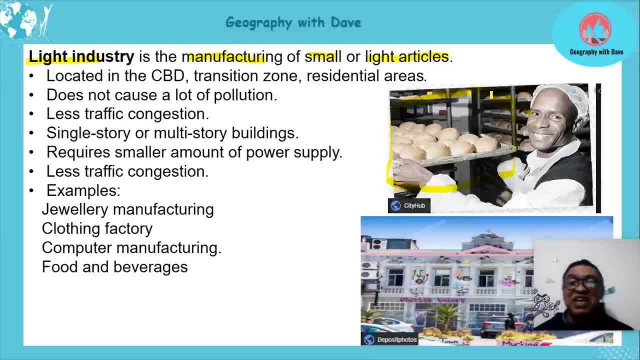 most probably that roads are smelling very nice. okay, so you can see that. all right, it's more light stuff. it can be located in the cbd transition zone residential areas. it doesn't have to be on the outskirts. let's look at reasons now why it can be situated in all these places in the residential 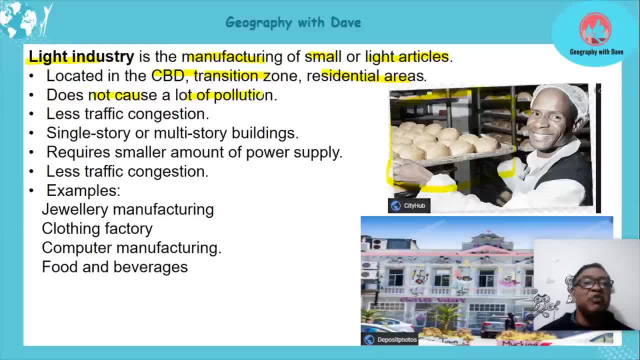 area. also, it does not cause a lot of pollution. okay, there's not much pollution. that's caused a bit of it, but not like as i showed you, with those tall chimneys giving off this because there's so much bug processing, etc. less traffic congestion. you know the bakeries will use vans. 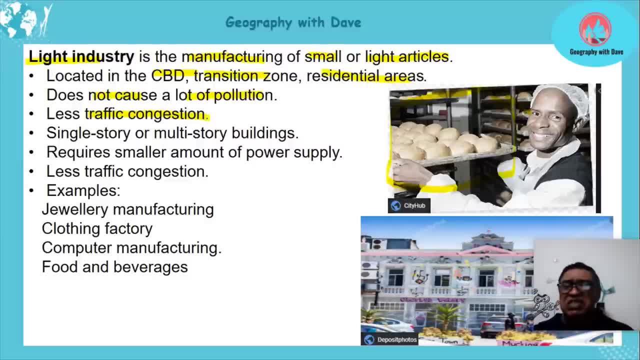 etc. the tailor shop will use things that are not, uh, not huge vehicles. okay, uh, it's. it can be single story or multiple story. you can have a light industry, all right, like a tailor shop on the second floor of a building. it's not parking. goods etc. requires a smaller amount. 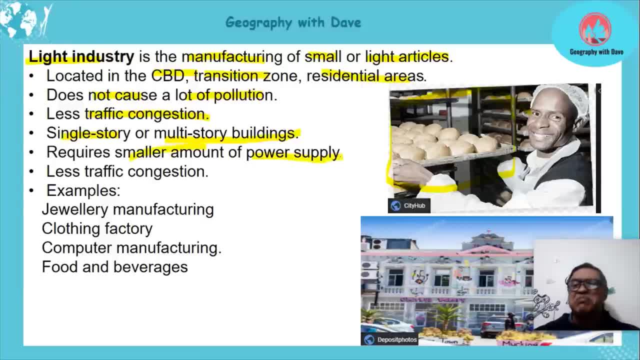 of power supply. you don't need massive things. there's no massive furnaces and whatever that you need there. all right, i like less traffic congestion. i've repeated it here. okay, some examples. manufacturing: you don't need the clothing factories. okay, which could be your smaller? what can be your tailor shop, etc. computer manufacturing: okay, and food and beverages. 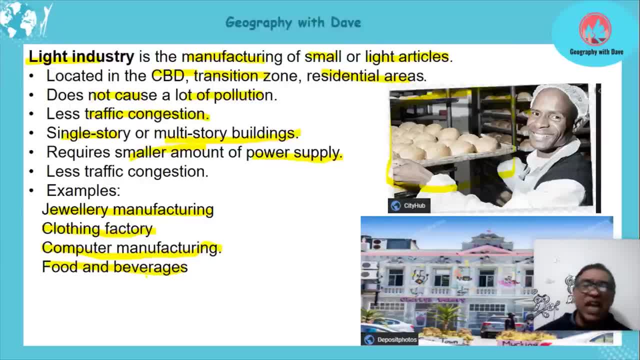 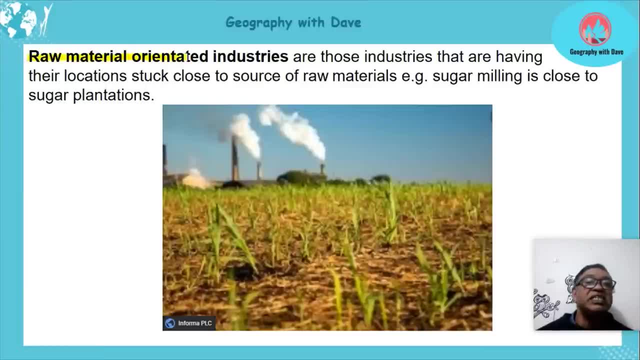 like your bakeries etc. massive their light industries. okay then, raw material orientated. it gets the meaning from that. raw material orientated. already you can work it out: are those industries having their locations stuck close to the source of raw materials. example: a sugar milk close to the sugar plantations. 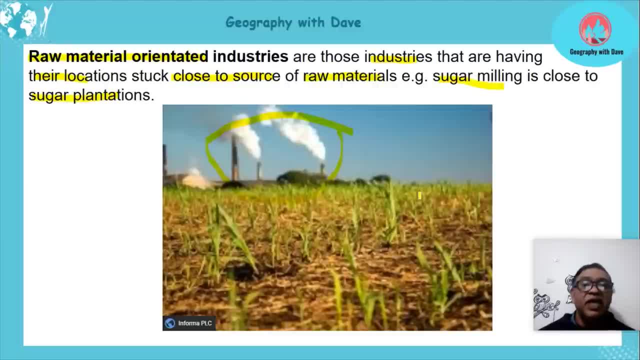 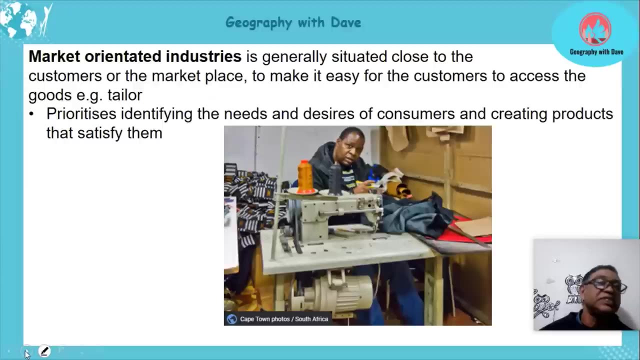 there's your sugar, yeah, right, okay. and there's your sugar plantation here. can you see it's carrying all this sugar cane, etc. market's right next door, okay to that, so you can process it right there. okay, we then have market orientated, generally close to the customers. 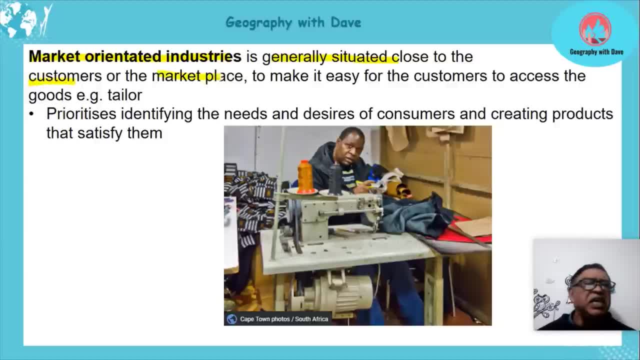 and or the marketplace. a reason there: it actually makes it easier for customers to assess or access the goods. example: a tailor: all right, it prioritizes identifying the needs and and desires of the consumers. it's based on that, you understand. okay, creating products to satisfy them. okay, to satisfy them. so they will create things based on the desires and needs. 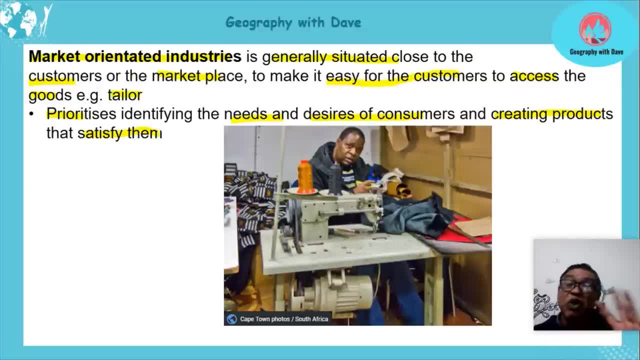 i know you go to a tailor shop and you want your clothing in a certain way. you understand it's there, it's next to the market. if there's no market, you understand this poor guy won't have a shop. so it's market orientated. it needs to be near the market, you understand, so people will. 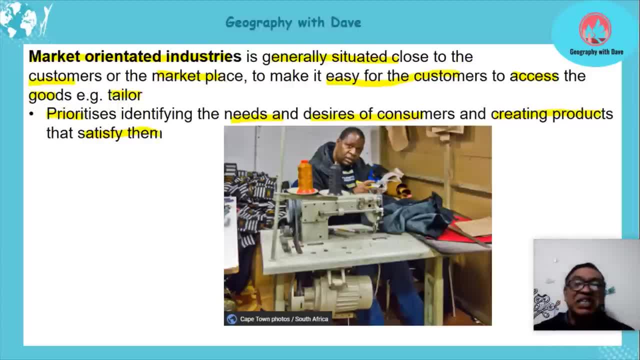 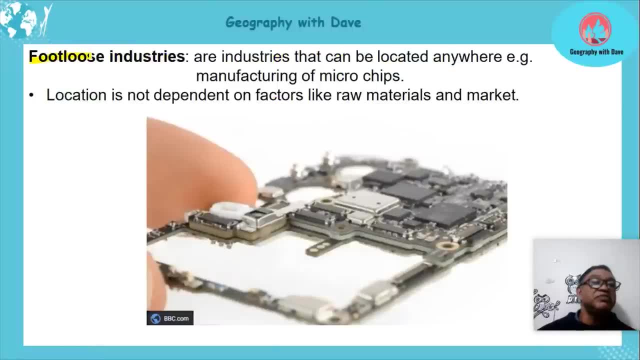 come in and assess- okay, based on their needs and, of course, desires. okay, footloose industries- now there's something about this industries. they can be located anywhere. example: manufacturing of microchips. these are light things. if you look at the guy's finger here, oh all right, he doesn't have that big fingers. it looks big because a microchip is a small thing. 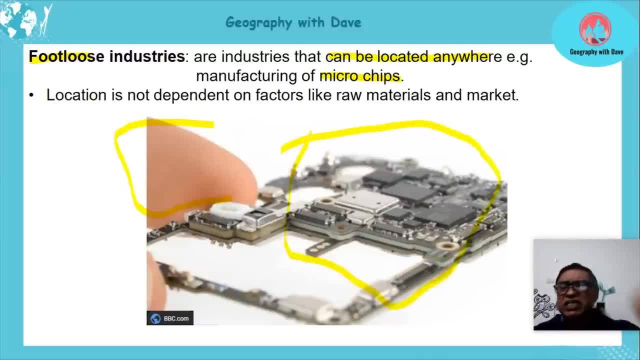 you understand, so it can be produced anyway. it doesn't have to be next to the raw material, it doesn't have to be next to the market, as i said here, not doesn't have to. not dependent on raw material and market or interior. not orientated means that it does depend on raw materials to 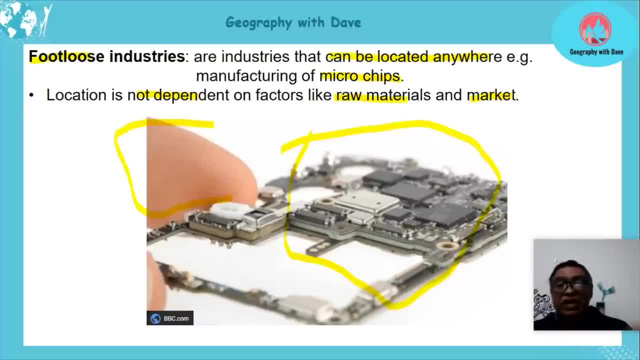 produce it, but doesn't have to be near the raw material or near the market. so we must. i must actually emphasize that it's not dependent on being near the market or raw materials. apologies, but i think i've rectified it because it doesn't need to. it deals with small quantity of raw materials. it's light products. you. 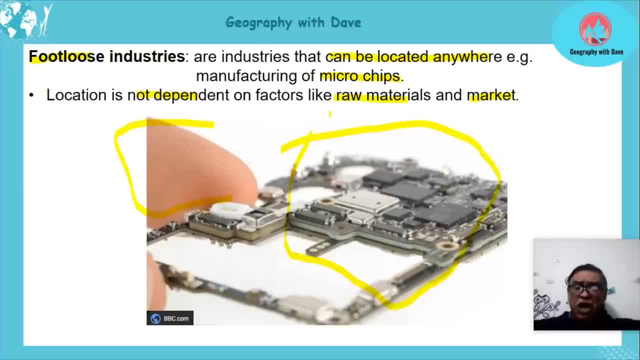 can have it away from the market. you can take a bulk, a lot of computer chips put into your boot and you can take it to the market all right. so it's not like heavy bulky goods. so it does remember again, footloose industries do not have to be near the raw material or the market. okay, it can be anywhere and it's fine. just 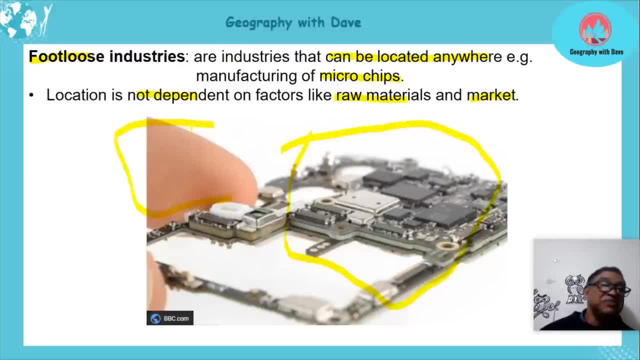 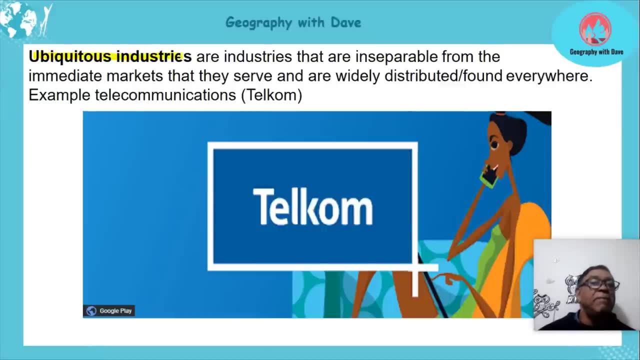 transported in a car or whatever. okay, then let's take an ubiquitous. i've got it right now, ubiquitous. i always have a problem. in fact, in class, the learners laugh at me also. who pick your test? fantastic, dave, well done, all right, uh, with you, just in this case. now we must be very careful here. 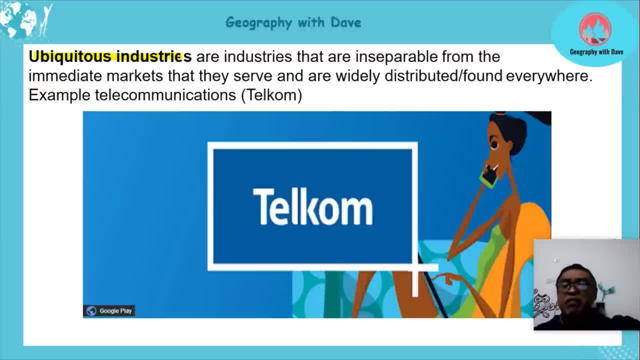 footloose doesn't have to be near the market, near the raw material- okay, but small products. here we have industries that are inseparable from the immediate markets. they serve- okay. so they need the market- all right, they need the market, but they are widely distributed- all right, they are widely distributed and found everywhere. now what am i saying here? 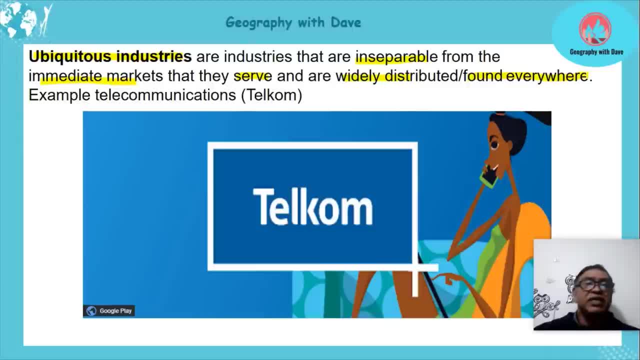 okay, i'm saying there's a difference. all right, let's just take the example of telecommunications. telecom, all right. okay, now telecom can be found anywhere. okay, they set out the internets, they set out the wires, the fiber, the whatever, all right, and they put it there. it can be found in the 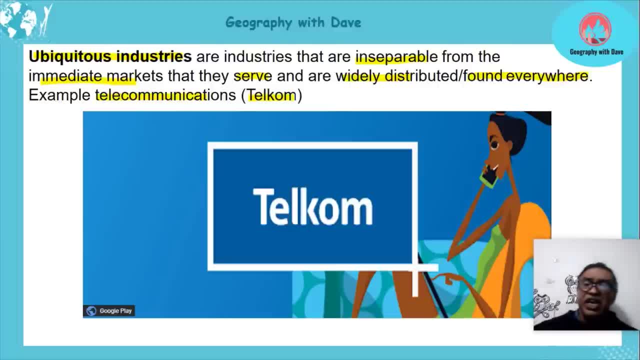 industrial area. it can be found in a residential area, all right, it can be found in a business sector. even if you take not land use zones but land use like recreation, you will find sometimes the systems are working through. okay, we all would agree with that. but there's a difference. okay, if there's no market, nobody wants it. let's take an internet connection. 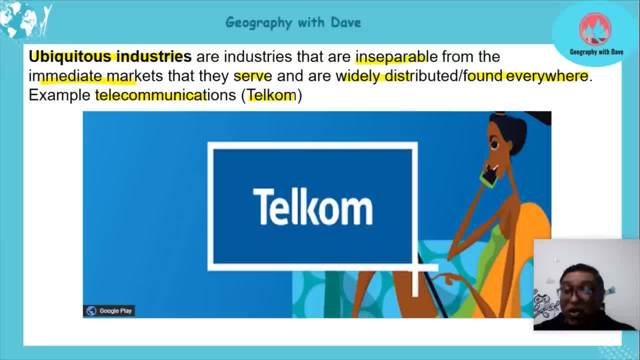 or telecom, etc. or their lines and things, then they're not gonna put it there, you understand. so it's around everywhere. it can be found anywhere, uh, chances are like a footloose industry, like a tailor shop, you understand, it's not dependent on the market, all right uh. but here this one is so. 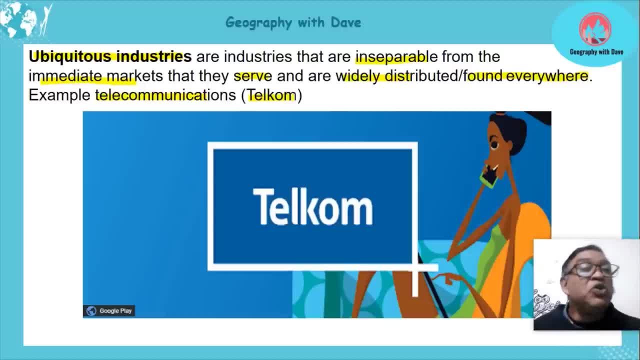 that is your difference between ubiquitous and footloose industry. it does. footloose does not have to be near the markets. you understand, here we find they are inseparable from the markets. it actually goes through the areas like: okay, I hope I brought out the difference between the two. okay, right, 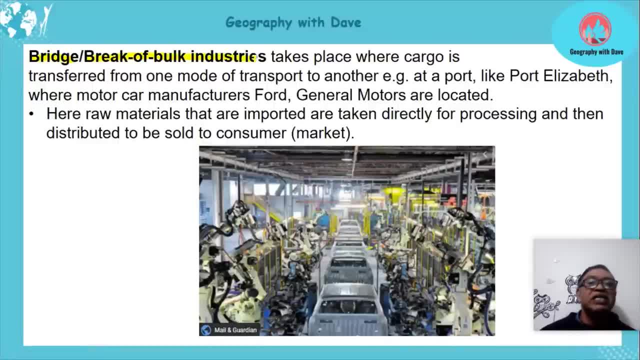 Bridge or break of bulk Industries. this takes place where cargo is transferred from one mode of transport to another. okay, that's where these Industries take place. example: Port like Port Elizabeth. okay, in South Africa, what happens here? we're car manufacturers, we're motor car manufacturers. you find Ford, General Motors, Etc. located. okay, so at this point it's very, very 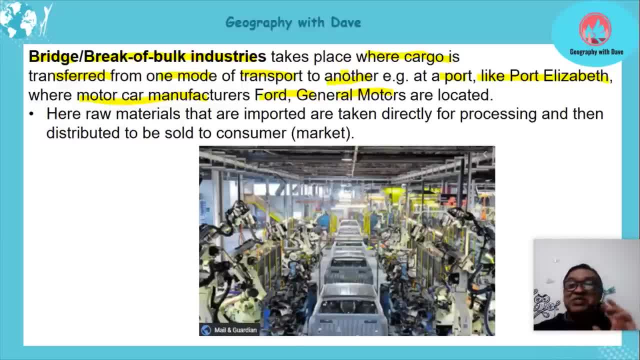 beneficial to these heavy Industries to locate there. because what happens? they may require some semi-process or raw materials or parts that come from other countries and they come to the port okay, and what happens at the port is they don't have further Transport costs, Etc. they take it directly into the factories or Industries. 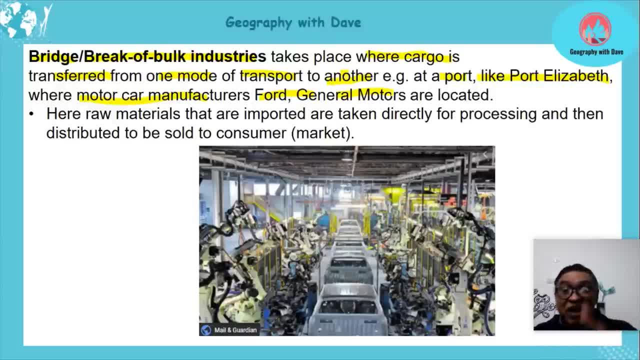 and the manufacture day, okay, and from there, when it's manufactured, it goes to the car sales, Etc. and then it's sold to the consumer, okay, or the market itself, okay, but that's where these Industries are situated. so, yeah, the raw materials are imported, all right, and taken directly for processing, because it's right at the part. 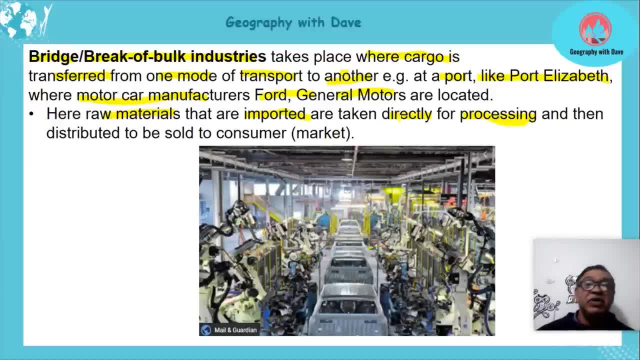 okay. so it's taken directly, saving a lot of course, okay- and then distributed to be sold to the consumer or market. it can be both ways. it can be then sold- you understand parts of it, then go off. the finished products go off into the country, to, let's say, Port Elizabeth, to Western Cape, to how dang Etc, or it can be exported you.